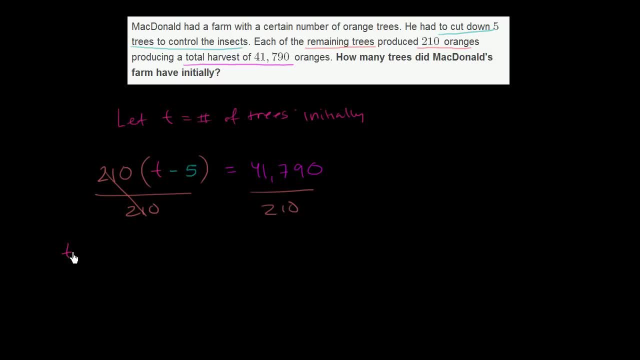 The left-hand side simplifies to t minus 5.. The right-hand side: let's see what is 4,000?. I'll do some long division here, I'll do it on the side. So 41,790 divided by 210.. 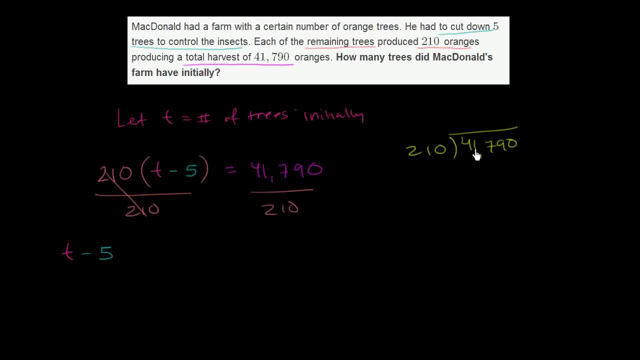 Let's see: 210 does not go into 4, does not go into 41. It goes into 417 one time, because two times would be 420. One time, 1 times 210 is 210. You subtract. 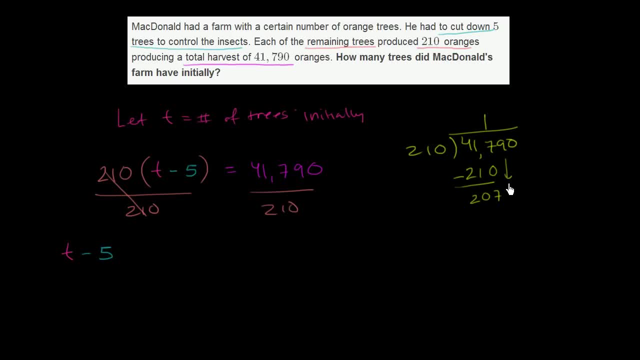 You get 207. And then you bring down the 9.. How many times does 210 go into 2,079?? It looks like it would go into it not quite 10 times. It looks like it would go into it 9 times. 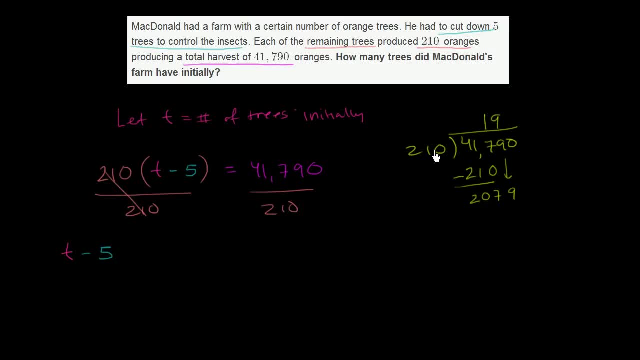 9 times 210 is going to be. let's see: 9 times 0 is 0.. 9 times 1 is 9.. 9 times 2 is 18.. And then we subtract. We subtract again: See: 9 minus 0 is 9.. 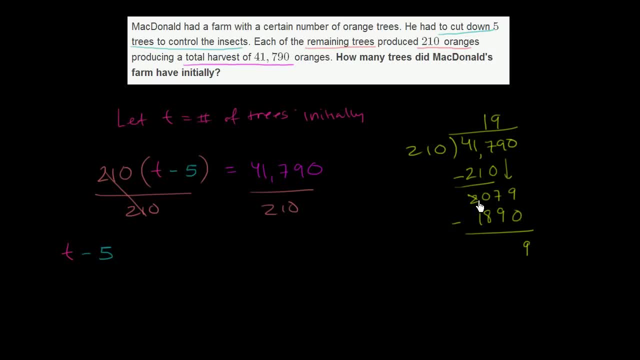 See, we have to regroup from the thousands place. So let's take 1,000 from there, Let's give that 1,000 to the hundreds place So it becomes 10 hundreds. But then we have to take 100 from the hundreds place. 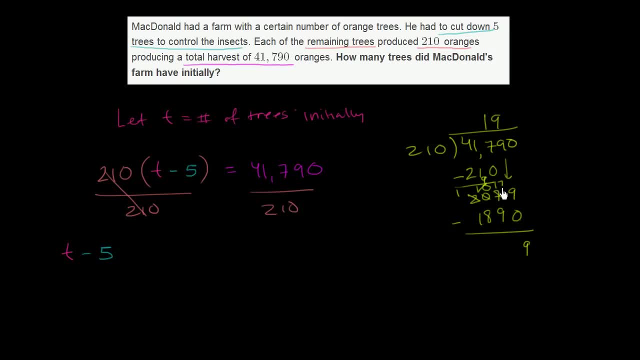 So this becomes 9.. And give it to the tens place, So this becomes 17 tens or 170.. So 17 minus 9 is 8.. 9 minus 8 is 1. And so we get 189.. 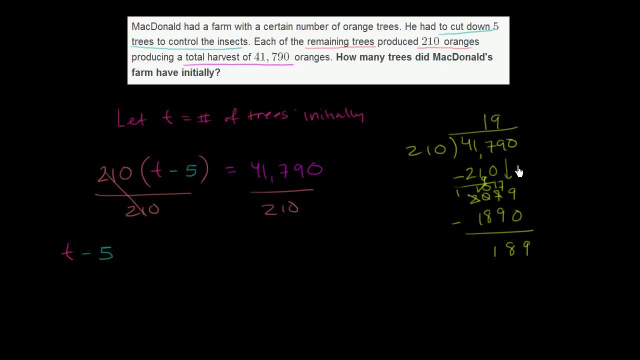 And now we can bring down another 0.. Bring down another 0.. It's a little off center right now And we already see that 210 goes into 1,899 times. 9 times 210 is 1,890.. 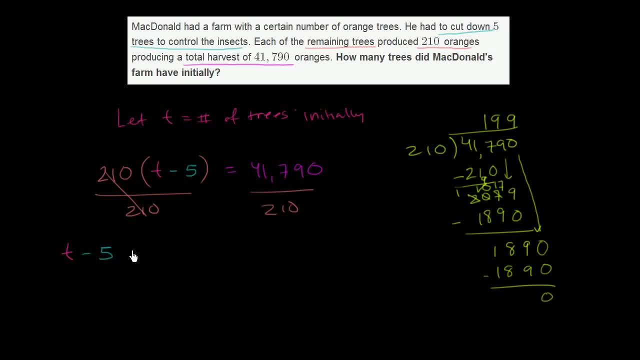 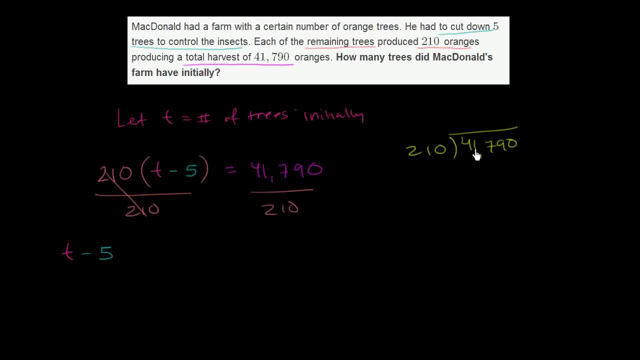 Let's see: 210 does not go into 4, does not go into 41. It goes into 417 one time, because two times would be 420. One time, 1 times 210 is 210. You subtract. 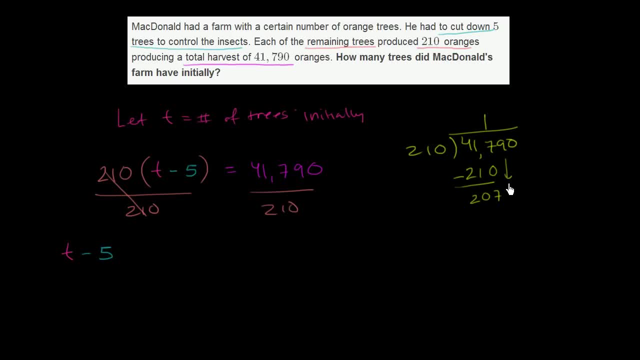 You get 207. And then you bring down the 9.. How many times does 210 go into 2,079?? It looks like it would go into it not quite 10 times. It looks like it would go into it 9 times. 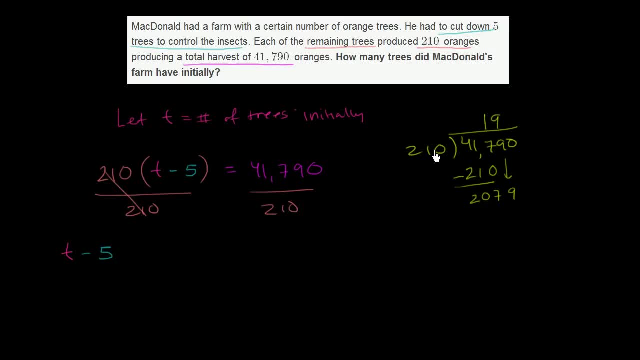 9 times 210 is going to be. let's see: 9 times 0 is 0.. 9 times 1 is 9.. 9 times 2 is 18.. And then we subtract. We subtract again: See: 9 minus 0 is 9.. 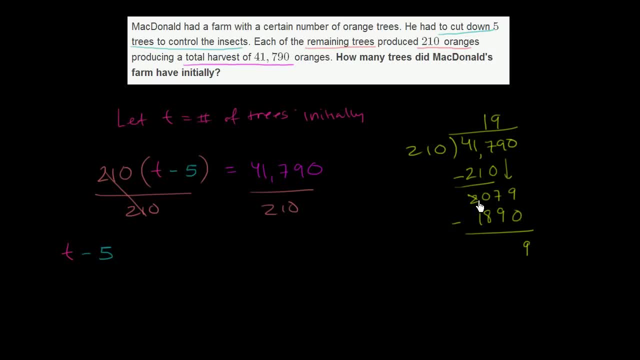 See, we have to regroup from the thousands place. So let's take 1,000 from there, Let's give that 1,000 to the hundreds place So it becomes 10 hundreds. But then we have to take 100 from the hundreds place. 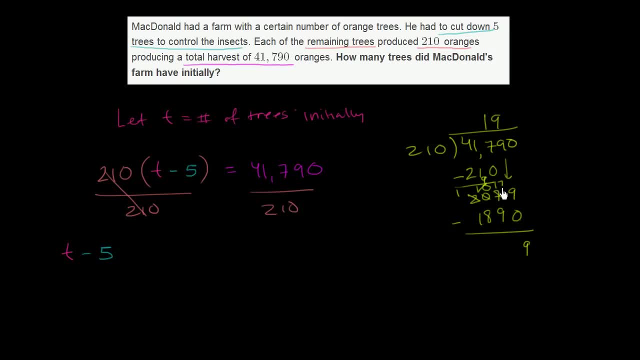 So this becomes 9.. And give it to the tens place, So this becomes 17 tens or 170.. So 17 minus 9 is 8.. 9 minus 8 is 1. And so we get 189.. 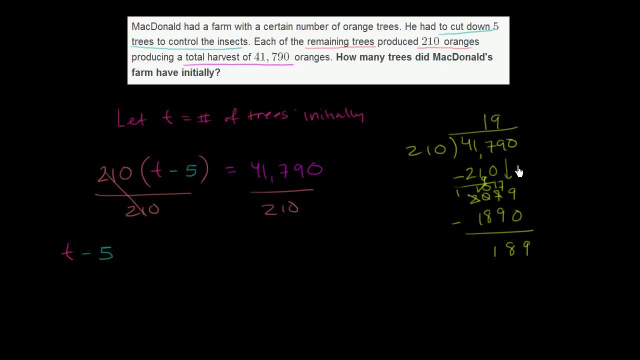 And now we can bring down another 0.. Bring down another 0.. It's a little off center right now And we already see that 210 goes into 1,899 times. 9 times 210 is 1,890.. 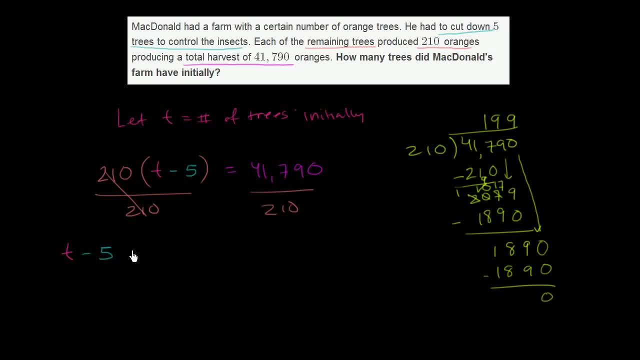 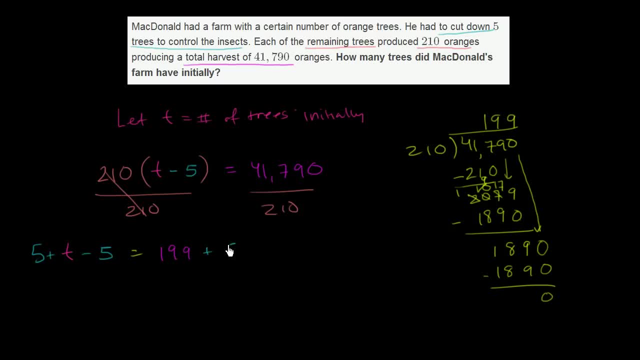 Remember, whatever we have to do to one side, we have to do to the other. Otherwise the equality wouldn't be equal anymore. They were equal before adding 5.. So if you want them to still be equal, you have to do the same thing to both sides. 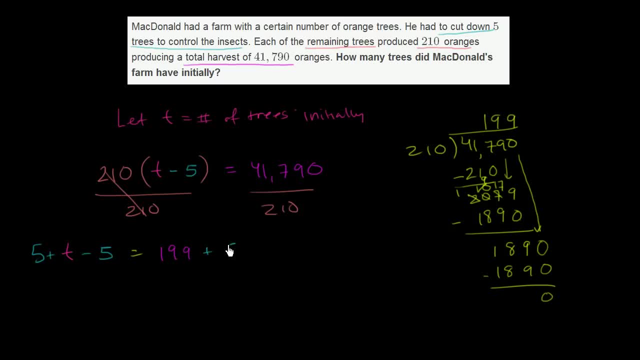 Remember, whatever we have to do to one side, we have to do to the other. Otherwise the equality wouldn't be equal anymore. They were equal before adding 5.. So if you want them to still be equal, you have to do the same thing to both sides. 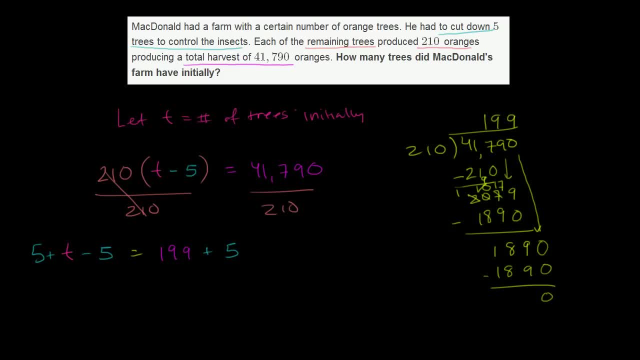 So the left hand side becomes T. The T in that purple color becomes T, And the right hand side becomes 204.. So he started off with 204 trees. Now I told you there's multiple ways to do this You could have, instead of dividing, 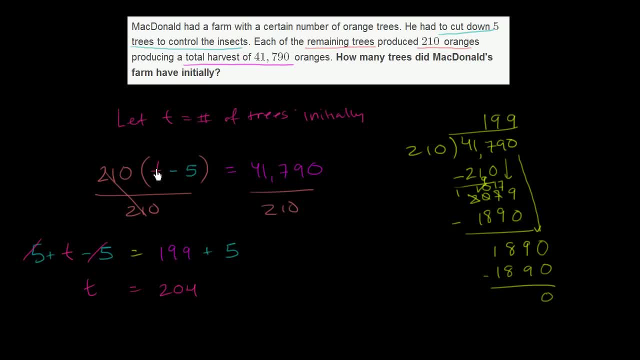 both sides by 210, you could have decided to distribute the 210. And then you would have ended up with- let me do another alternate way of doing it: 210 times T minus 5 times 210.. Minus 210 times 5.. 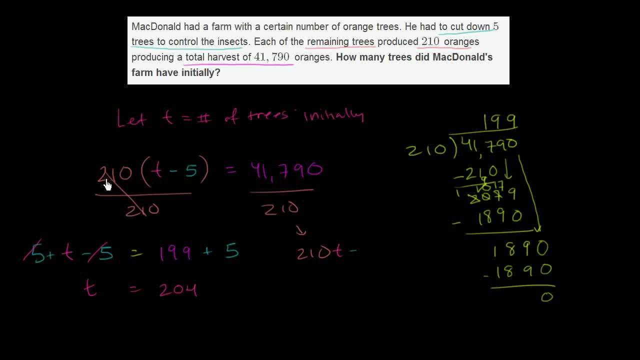 Actually, let me just multiply it out so we save some space. 5 times 210 is 1,050.. Minus 1,050. Is equal to 41,790.. And then you could add 1,050 to both sides. 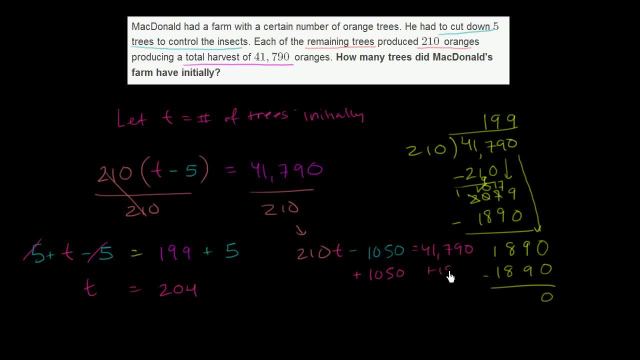 And so let me do that: 1,050 to both sides. 1,050, not 150.. 1,050 to both sides. The left hand side, you're just going to be left with 210 T, While the right hand side, you're going to be left with. 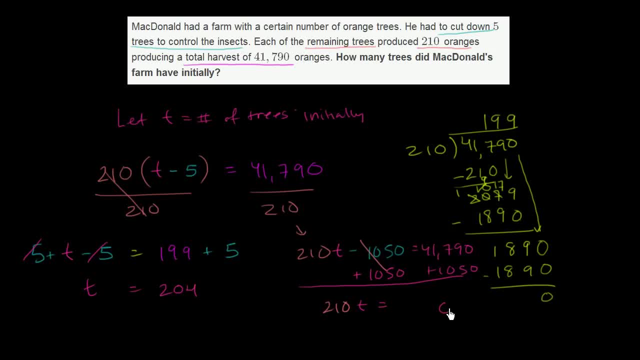 let's see you're going to be: 0 plus 0 is 0.. 9 plus 5 is 14.. 1 plus 7 is 8.. 42,840.. And now you can divide both sides by 210.. 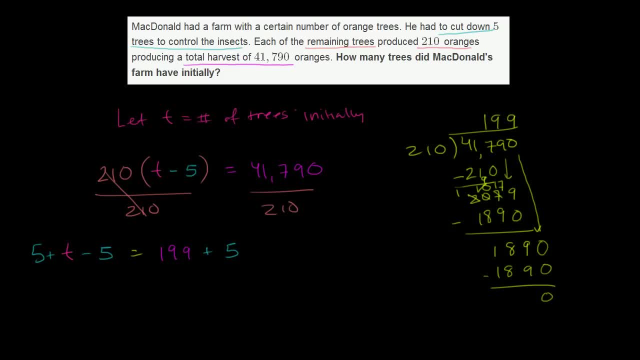 So the left hand side becomes T. The T in that purple color becomes T, And the right hand side becomes 204.. So he started off with 204 trees. Now I told you there's multiple ways to do this You could have, instead of dividing, 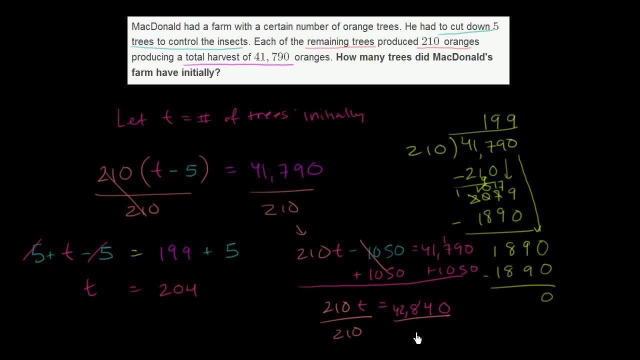 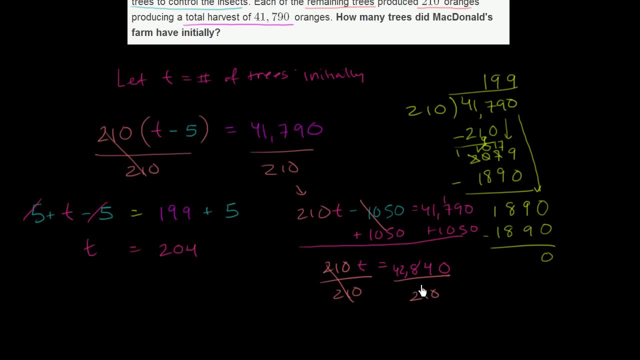 You could divide both sides by 210.. And now we know where this is going to go. I could do the long division again. T is going to be equal to 42,840 divided by 210, which is equal to 240. OK, OK Again. So I'm going to divide both sides. You could divide both sides by 240.. There's not going to be any difference between these two sides, And this is actually going to be equal to, all the way around, 1,045.. So the last two guys going to have to do the long division. Here's what I'm going to do, so I'm going to go ahead and divide both sides by 20, so 1,2.. 1,2,540.. And then I'm going to divide them down by 2,045.. And now I'm going to divide them by 2,2,520.. There's a little bit of a gap in there. Let's see.